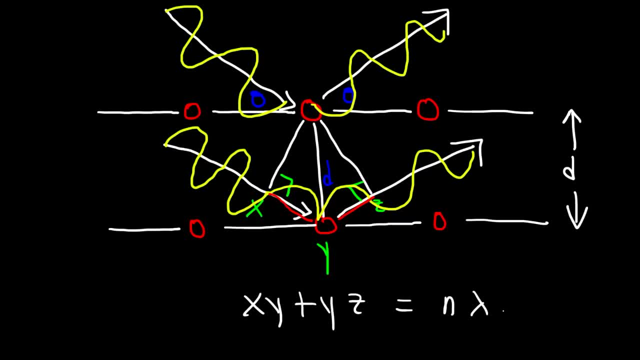 So it's going to be n times lambda, where lambda is the wavelength of the x-ray, And that can be 2 times lambda, 3 times lambda, 4 times it. It can vary, But if you're dealing with a problem that says first order, diffraction n is 1.. 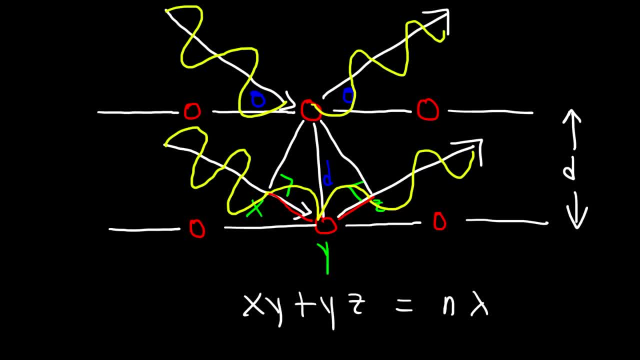 If it's second order, diffraction n is 2, and so forth. Now I'm going to go backwards. I'm going to rewrite this equation shortly, Because there's something else I need to show you Now. this angle that we have here is the same as this angle. 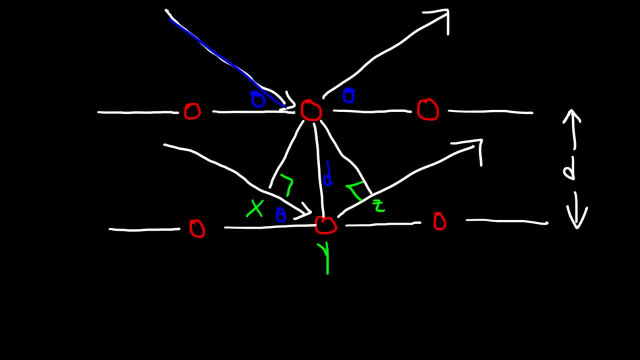 Because these two lines they're parallel, Or at least they should be parallel. My drawing is not perfect. And then this angle is the same. Now, what we need to realize is that this angle, theta, is the same as this angle here. And for those of you who are not sure, let's say, if we have a horizontal line which represents this line, 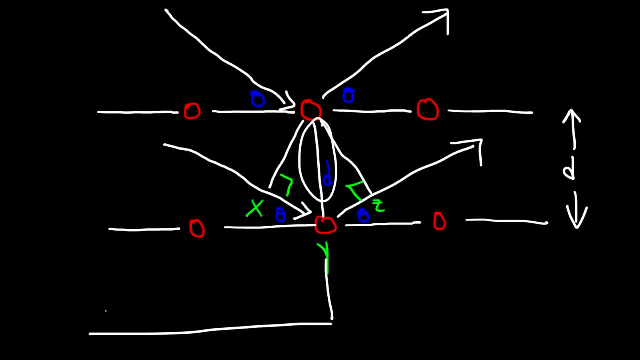 And then we have a line perpendicular to it, which is this line, And then we're going to draw a ray which represents this line, And then we're going to turn this into a right triangle. So let's say, if this is 30 degrees, 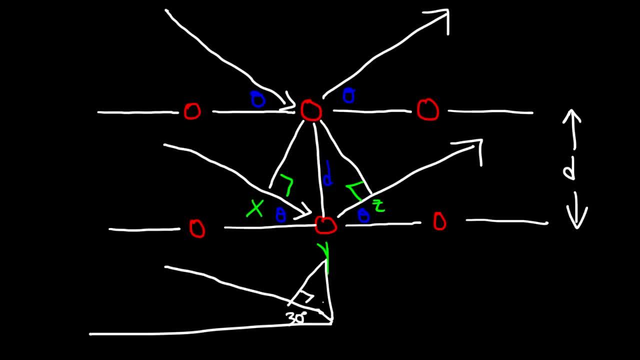 And this side is perpendicular to this side. That means this has to be 60. Which means this has to be 30. So, therefore, these two angles are congruent, They equal each other. So, therefore, this is theta And that is theta. 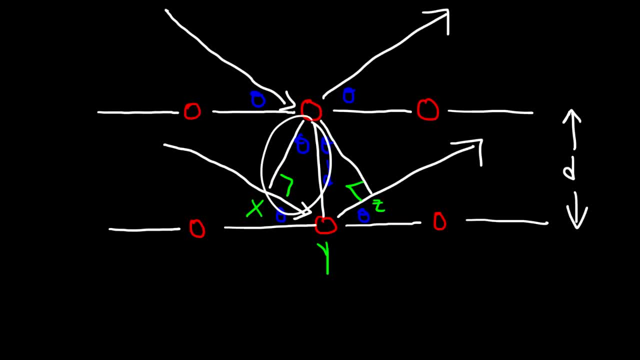 And that is theta as well. Now I'm going to draw just this triangle for now. So the hypotenuse of that triangle is d, as you can see here, And this side is xy, That is the distance between position x and position y. 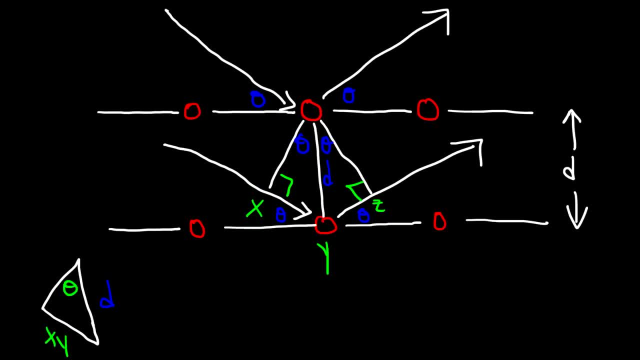 And then we have the angle theta. Now, using Sokotoa trig, we know that sine theta Is equal to the side opposite to it, which is xy Divided by the hypotenuse which is across the 90 degree angle. 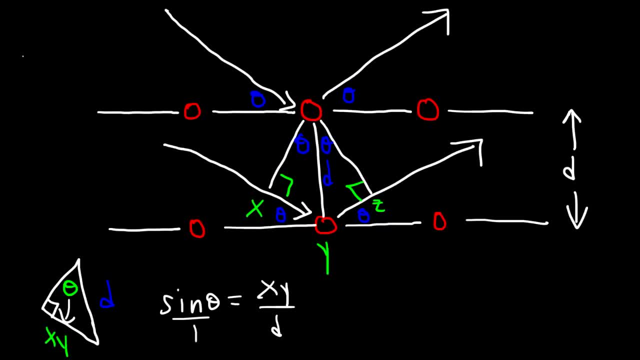 And that's d. So if you cross, multiply, you'll see that xy is equal to d sine theta. Now, if we focus on this triangle- Okay, that was a messed up drawing, Let's do that again- Here we have the angle theta. 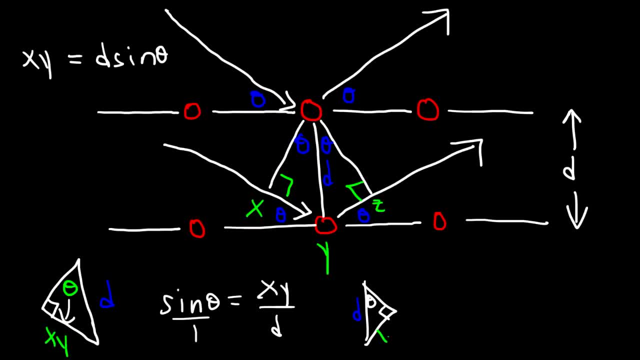 This is d, And then this side is yz. So sine theta is equal to the opposite side, which is yz, Divided by the hypotenuse, which is d. So cross multiplying, we can see that d sine theta is equal to yz. 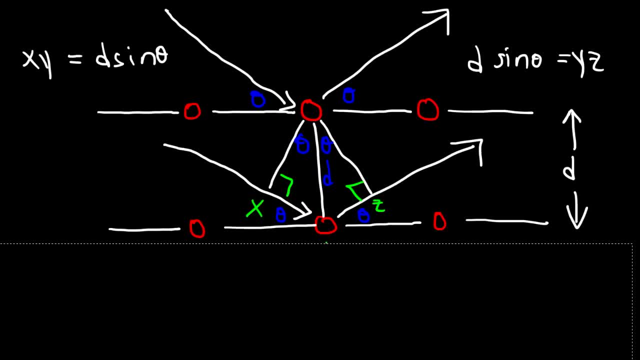 Now let's go back to the other equation that we had before. Well, we said that xy plus yz is equal to n times the wavelength. So the extra distance that the second wave travels is xy plus yz, And that extra distance has to equal the wavelength or multiple of the wavelength. 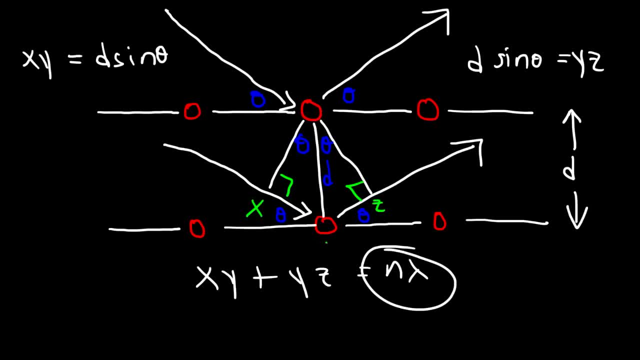 Which is n times lambda. Now let's replace xy with d, And that's d sine theta. And let's replace yz with d sine theta, So 1d sine theta plus 1d sine theta is 2d sine theta. 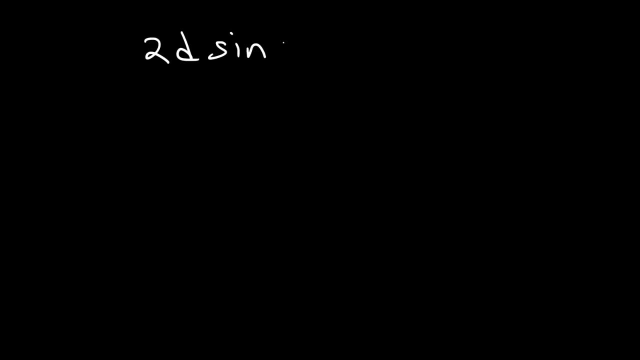 So now we have Bragg's equation, which is: 2d sine theta is equal to n times the wavelength, So this is the equation that we're going to use To solve this equation And to solve problems associated with Bragg's equation. 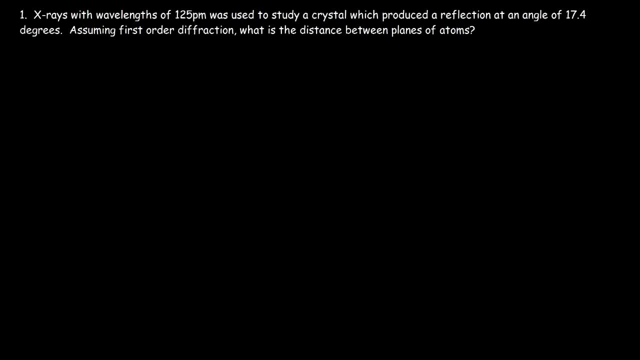 Let's start with this problem. X-rays with wavelengths of 125 picometers was used to study a crystal which produced a reflection at an angle of 17.4 degrees. Assuming first order diffraction, what is the distance between planes of atoms? 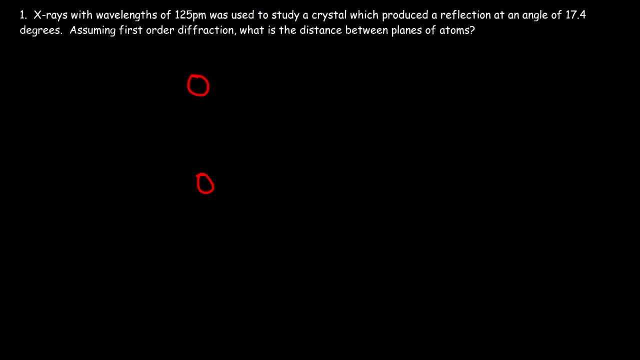 So let's draw a picture. So this is the distance that we're looking for, And here we have an x-ray that strikes an atom and then it bounces off, And it does the same thing to this atom as well. Now, the angle at which it strikes the atom relative to the x-axis, that's 17.4 degrees. 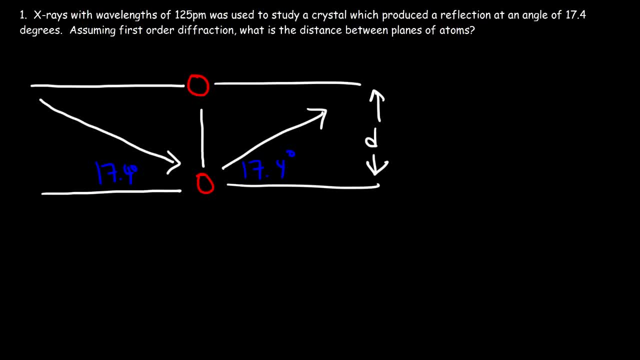 Which means this angle is the same. So that's theta And we have the wavelength. It's 125 picometers And assuming first order diffraction. so n is 1, we need to calculate d, So therefore we can use this equation. 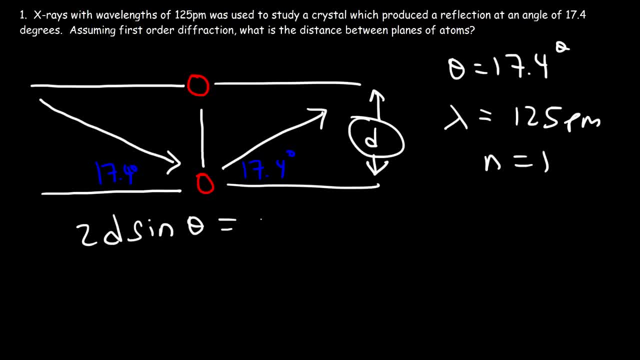 2d sine theta is equal to n times lambda. So solving for d, we need to divide both sides by 2 sine theta. So n lambda divided by 2 sine theta Is equal to the distance between the planes of atoms. So in this example n is 1.. 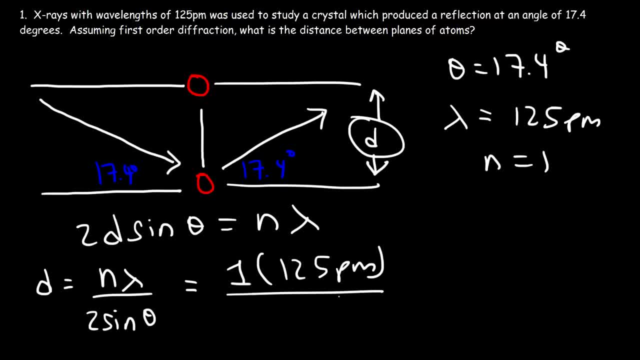 Lambda is 125 picometers Divided by 2 times sine of 17.4 degrees. So let's go ahead and plug this in, So you should get 209 picometers. So that is the distance between the planes of atoms. 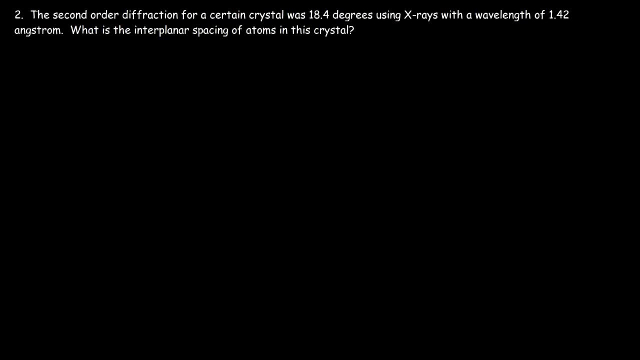 Now let's move on to the next problem, Number 2.. The second order diffraction for a certain crystal was 18.4 degrees. using x-rays with a wavelength of 1.42 angstroms, What is the interplanar spacing of atoms in this crystal? 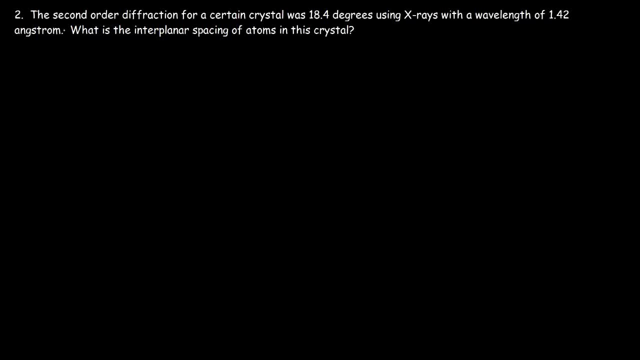 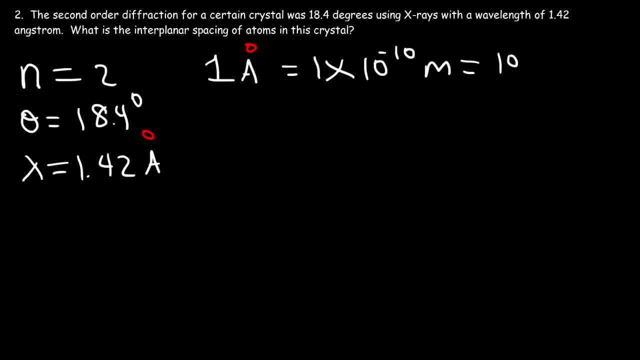 1 times 10 to the minus 10 meters, Which works out to be 100 picometers. So now our goal is to calculate the interplanar spacing of the atoms in this crystal. So we're looking for d, So we can therefore use the same equation where d is n multiplied by lambda, which is the wavelength. 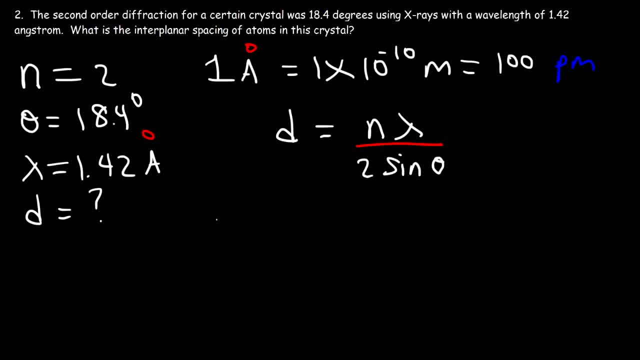 divided by 2 sine theta, So n in this example is 2.. Lambda is 2. And lambda is 1.42 angstrom. And let's divide that by 2 sine of 18.4 degrees So we could cancel 2.. 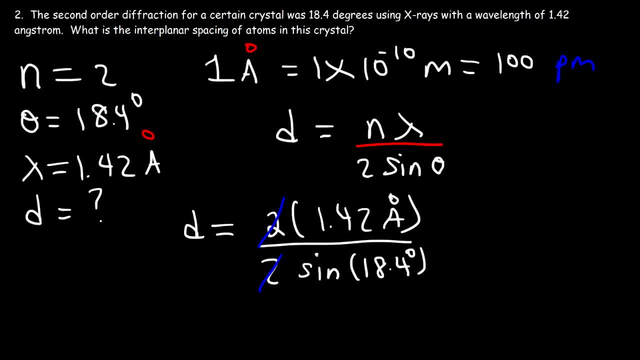 2 divided by 2 is 1.. Now if lambda is in angstroms, d is going to have the same unit. So if we take 1.42 and divide it by sine- 18.4,, we get 1.42.. 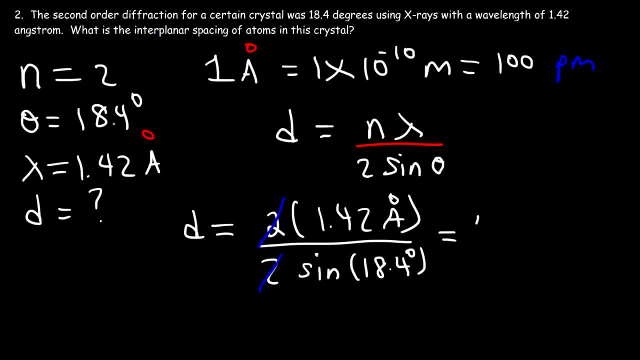 This is going to be 4.50 angstroms, So that's the distance between planes of atoms in this crystal. Now let's convert that to picometers. 1 angstrom is 100 picometers, So 4.5 angstroms is going to be 4.5 times 100, which is 450 picometers. 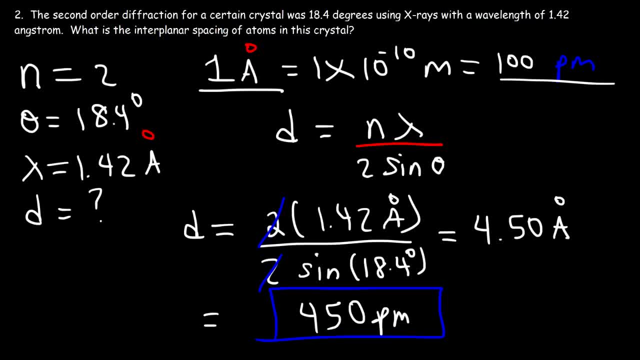 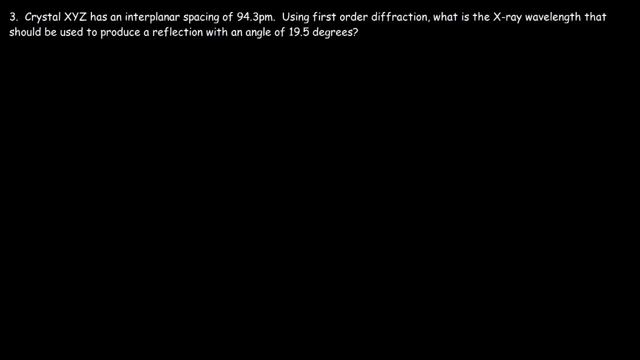 So that's the interplanar spacing of atoms in that unit, Number 3.. Crystal XYZ has an interplanar spacing of 94.3 picometers. Using first-order diffraction, what is the X-ray wavelength that should be used to produce a reflection? 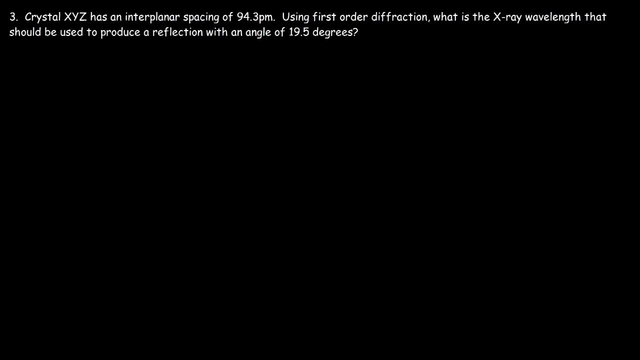 with an angle of 19.5 degrees. So in this example we have the distance between the planes of atoms, So that's d And that's 94.3 picometers. Now we're dealing with first-order diffraction, So n is 1.. 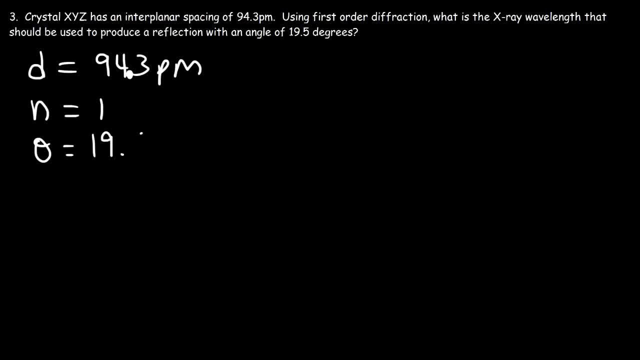 And the angle is 19.5 degrees. What is the X-ray wavelength? So we're looking for lambda in this problem. You can pause the video if you want to try it. So let's start with this form of the equation: 2d sine theta is equal to n times lambda. 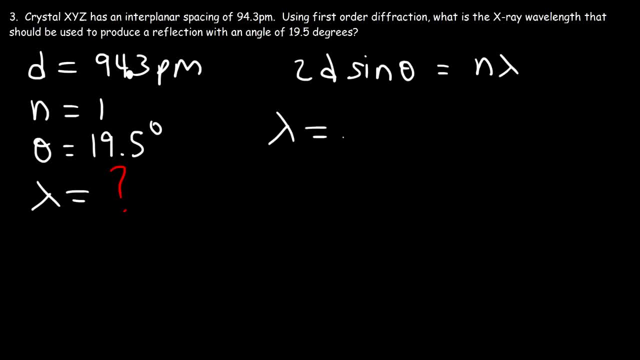 So if we divide both sides by n, the wavelength is 2d sine theta or over n. So that's going to be 2 times 94.3 picometers multiplied by sine of 19.5 divided by 1,. 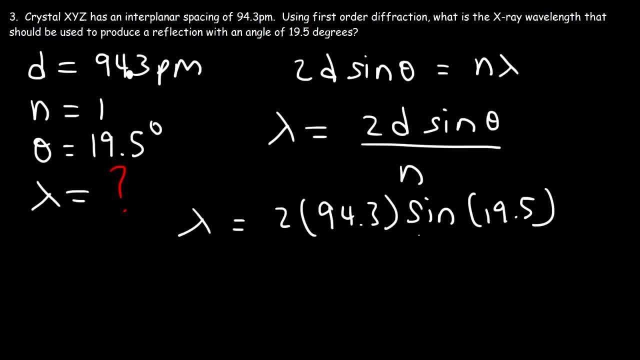 which, when you divide something by 1, it's not going to change. So the answer that you should get is 62.9.. So the answer that you should get is 62.96 picometers. So make sure that these two share the same unit. 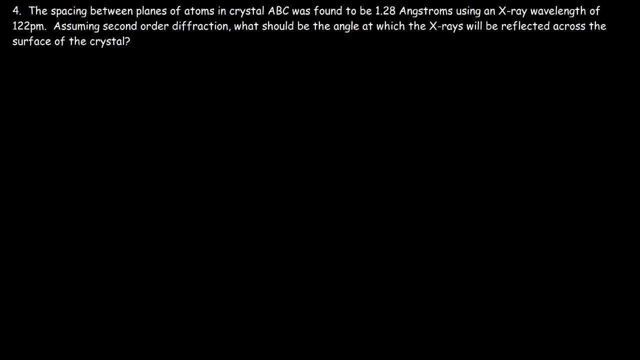 And that's it for this problem. The space in between planes of atoms in Christo, ABC, was found to be 1.28 angstroms using an X-ray wavelength of 122 picometers. Assuming second-order diffraction, what should be the angle at which the X-rays? 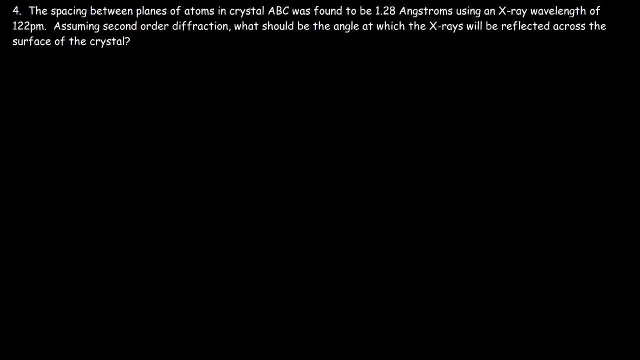 will be reflected across the surface of the crystal. So the space in between planes of atoms is D, That's 1.28 angstroms, And the wavelength is 122 picometers. So we need to make sure that these units match in order for this equation to work. 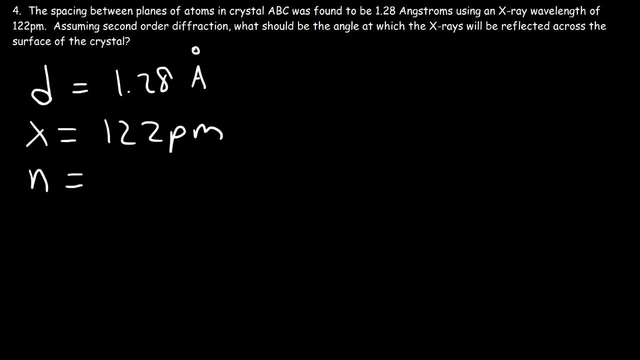 Now we're dealing with second-order diffraction, so n is 2, and our goal is to calculate the angle. So we're going to do that. Now we know that one angstrom is 100 picometers, So 1.28 angstroms must be 128 picometers. 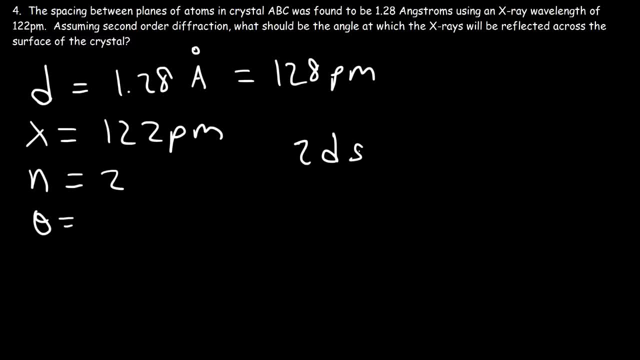 So now we could use the equation: 2D sine theta is equal to n times lambda. So let's divide both sides by 2D. So sine theta is n lambda over 2D. So that's going to be: sine theta is equal to n. 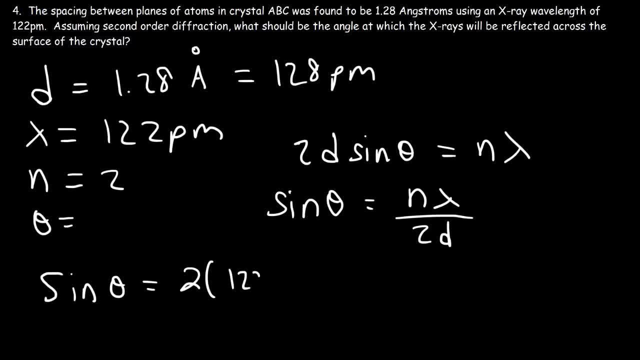 which is 2.. Lambda is 122 picometers And D is 128.. So 2 over 2 is 1.. So sine theta is going to be 122 divided by 128.. And so that's going to be 0.9531. 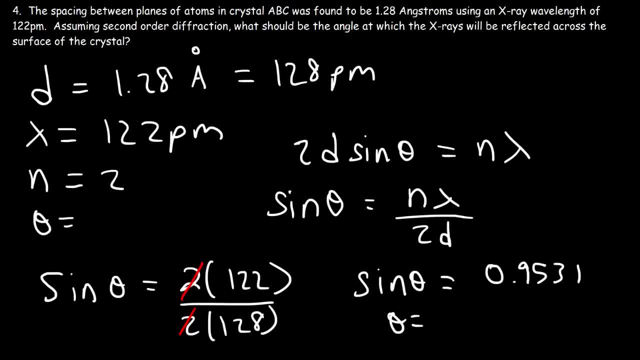 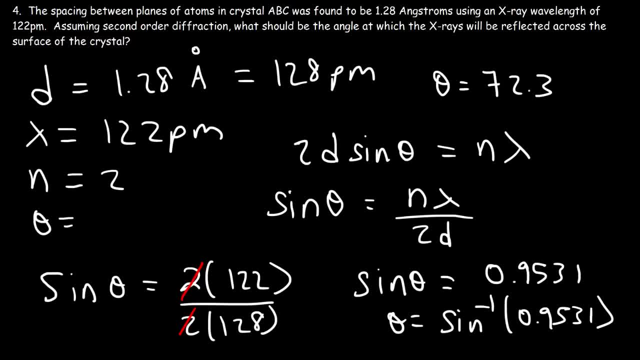 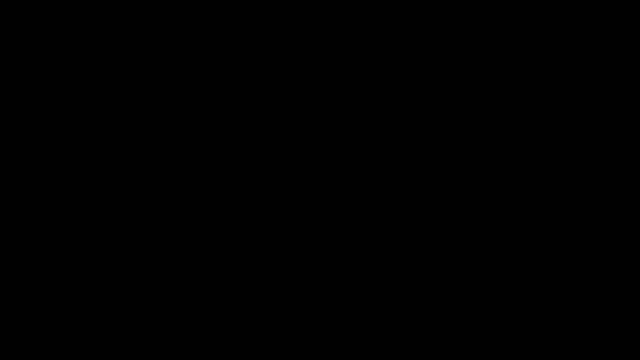 So the angle is 72.38 degrees And that's the answer to this problem. So now we're going to use the equation to find the angle theta. So we're going to use the equation to find the angle theta.